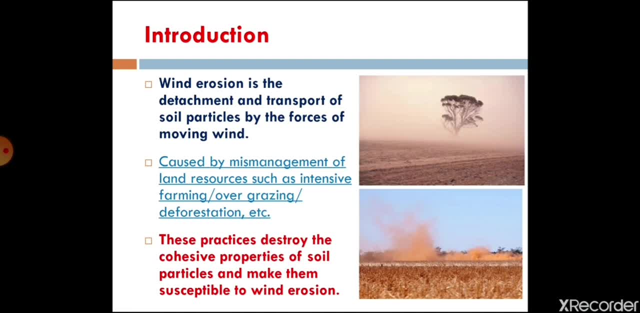 barren without any protective cover and due to no protection over on the earth surface. what will happen? the sun and, due to climate or high temperature, the moisture has gone. The moisture will gone from the soil surface and slowly, slowly, it will become dry and when it will become dry, the chances of wind erosion become high. 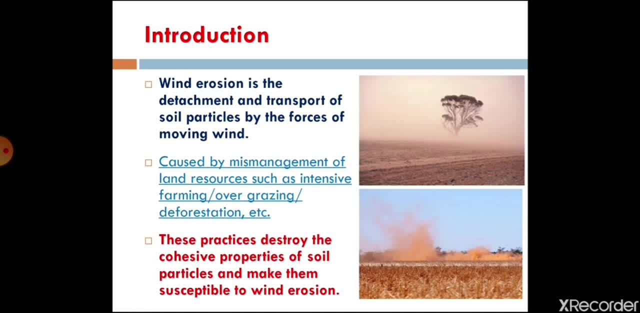 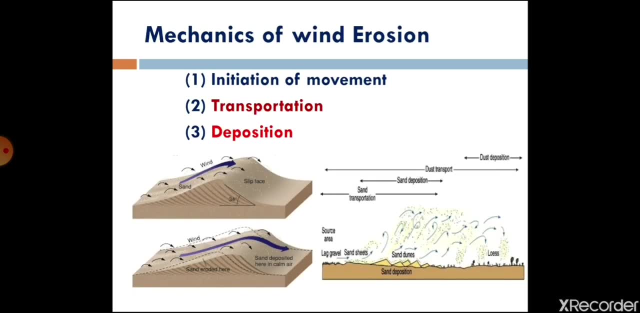 So, due to temperature and such kind of practices also, it also destroy the cohesiveness property of the soil. So if you see, there are three mechanics involved into the wind erosion. First one is initiation of moment. Initiation of moment means detachment of soil particle from the surface Just a minute. 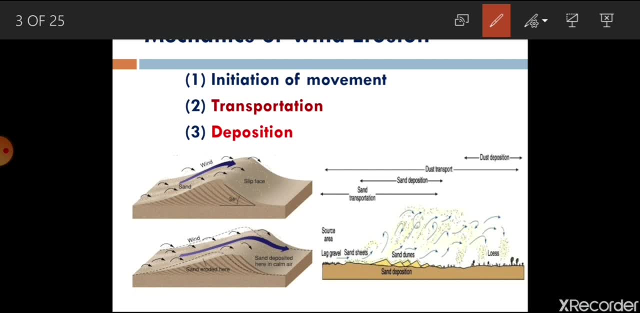 In contribution to this. we can see here. See, these are the soil particle which are moving. Okay, These dots. So it is a detachment of particle In initiation of movement, it is a detachment from soil surface. And then transportation – due to the action of wind or due to force of air. when such decided particles are moving ahead, they comes under transportation. 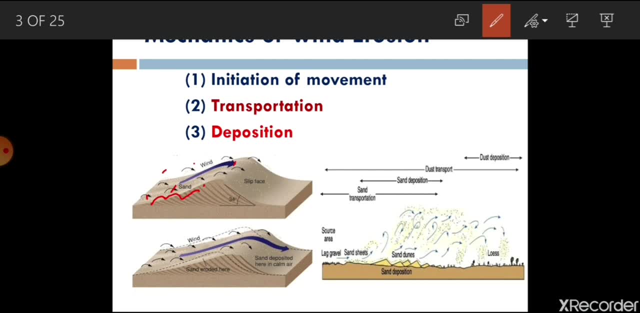 There comes under transportation And when wind develops, wind are getting expressed and physical part is getting. what called as kinetic particles is, for example, if wind velocity is lesser or obstructed by some barrier. if wind velocity is going like this and it is obstructed by some barrier or its 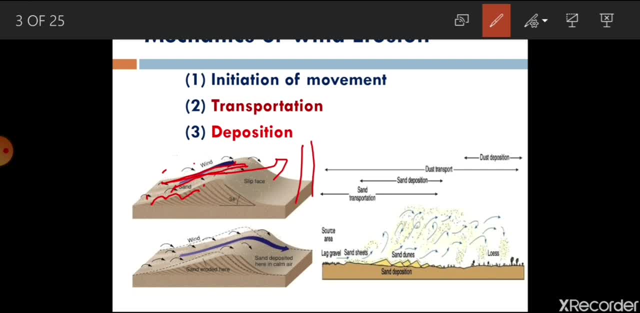 speed is, you can say, becoming little, low, slow. so what will happen? that whatever soil particle it is carrying, it will drop somewhere here. okay, so this is stuck here. deposition starts. so this is how these three moment are involved in wind erosion, initiation of moment, transportation of soil and deposition of 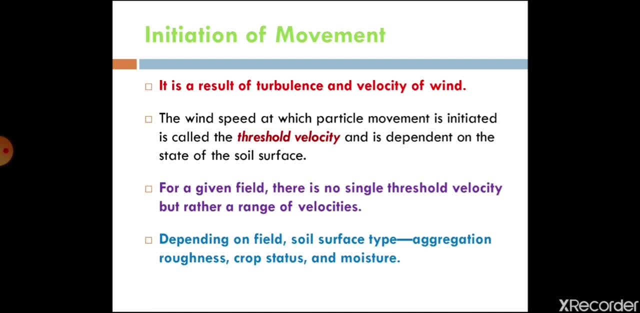 soil. so in detail we will discuss here initiation of moment created due to, or you can say, detachment of soil particle is created due to turbulence and high velocity of the air and when you know that complete field condition or soil condition are not uniform. so for a detachment of different soil particles there is 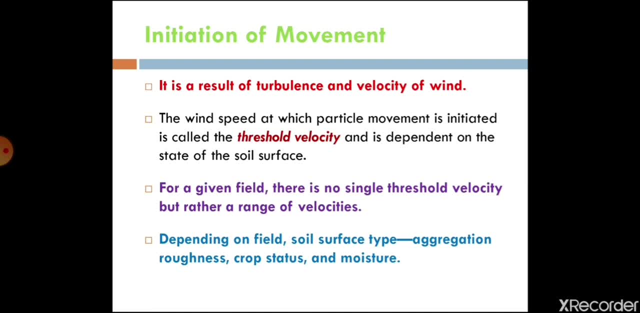 different velocities required, variable velocities required. so wind speed at which particle moment is initiated is called threshold velocity and I told you it could not be uniform. so there are velocity, there are various velocities for, say, in same field one particle may be removed or one particle may be. 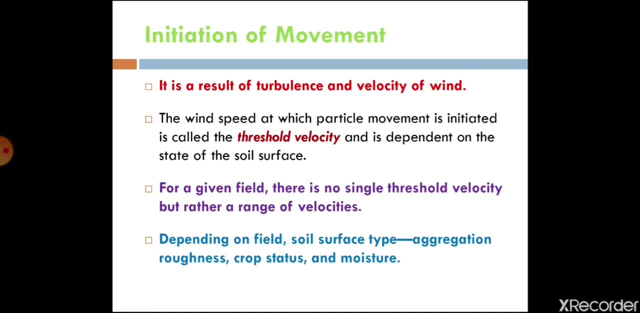 detached from different threshold velocity, whereas another particle will remove it. different threshold velocity so as a complete field condition may destroy or may get, may get affected by wind erosion due to variable velocity. so there are range of velocity, you know. you can say there are threshold velocity, variety of threshold velocity. 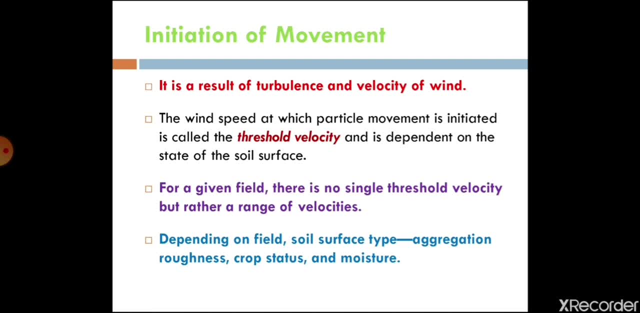 for a particular field. and apart from these velocity, the wind erosion, also affected by the surface type, whether surface type, surface type surface is rough crop is there on field or not? moisture condition: how much moisture condition is available. whether that moisture condition is able to hold the soil particle. 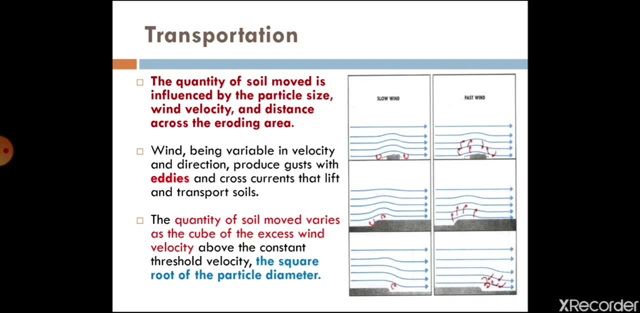 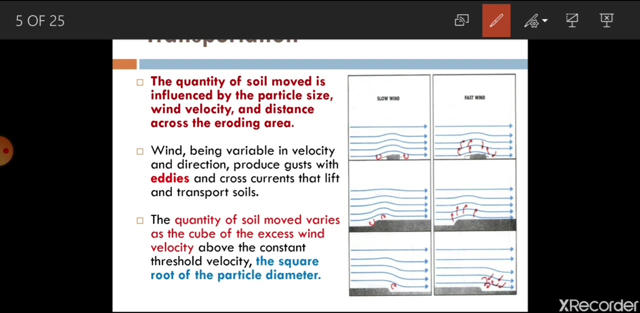 or not, that is adhesive property and cohesive property of the soil. Now coming to the next phenomena, that is transportation. So you see here in the diagram, particularly as you know, that transportation of soil particle depends on the size of particle and wind velocity. So when wind is moving uniform here and now, if some particle comes in between the wind, 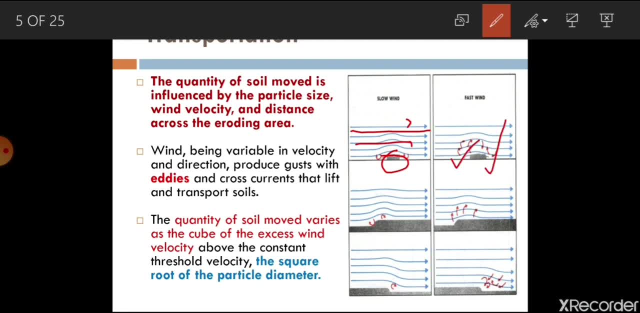 So what will happen? You see here, Some turbulence is created very near to the that object. or you can say that object may be rock, may be any vegetation or may any kind of things, So that rocks intercept the, or you can say reduce the velocity. 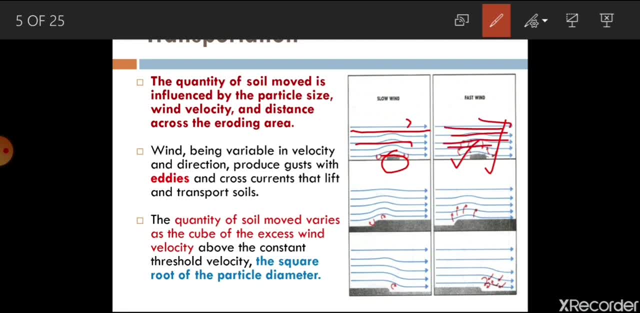 But the upper velocity, upper wind are moving at their pace. But at this particular point, at this object, Turbulence is created because it is objecting the flow of wind and due to this turbulence soil particle here are supposed to lift, And that quantity of soil moved varies as per the cube of excess wind velocity above. 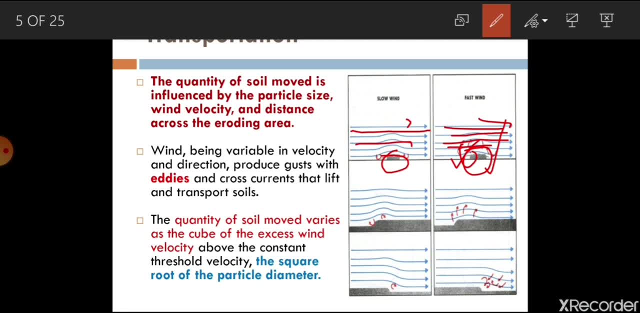 the constant threshold. So any kind of object, Either symmetrical object like here, Or Some projected object like this, And here you can see wind is moving here and when it is obstructing, this turbulence is creating and, due to this turbulence, soil particle or detached particle are lift into. 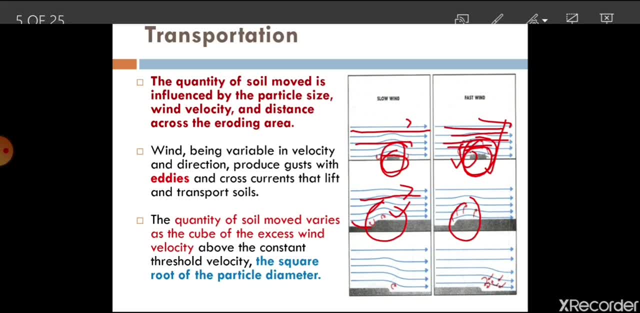 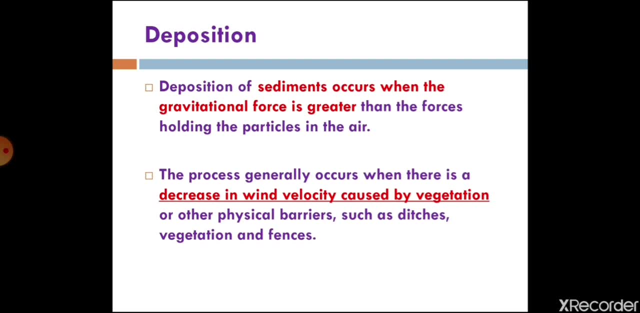 the velocity and it is moving ahead with the wind. Now, deposition after initiation of moment transportation of moment deposition. deposition occur Where gravitational force is higher than the wind forces, or you can say, when wind forces become weaker, The gravitational force attract the soil particle which is flowing along with the wind and it. 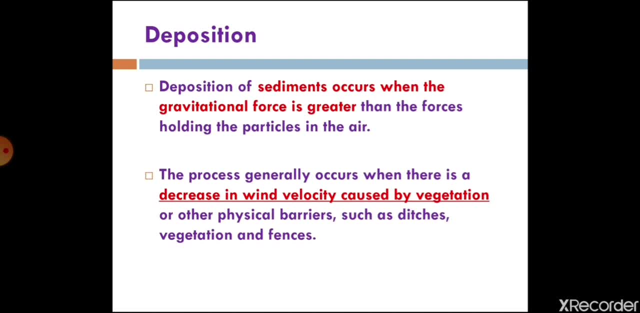 will drop at to particular point, So that particular point will known as deposition And not only the gravitational force. apart from, or you can say along with, gravitational force, there are few other parameters, there are few other things which can reduce the wind velocity, Say if some vegetation is coming. 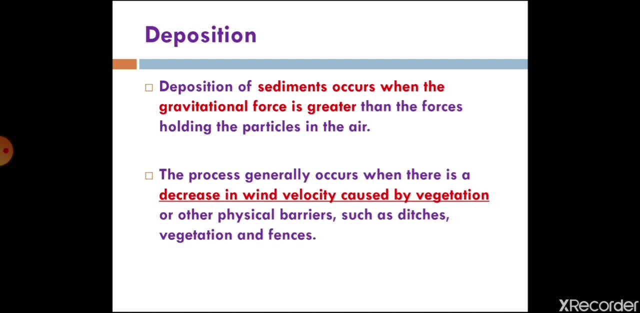 Some fields are well protected by the plants. so when? or any physical barrier is there, So when? So when? So when wind is flowing through the physical barrier or just striking the physical barrier, its velocity will reduce and once its velocity will reduce, the its capacity to hold the soil particle will. 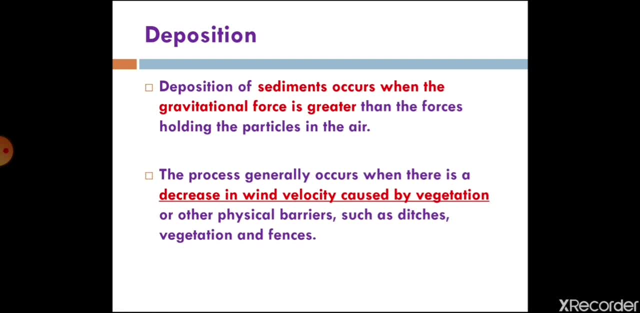 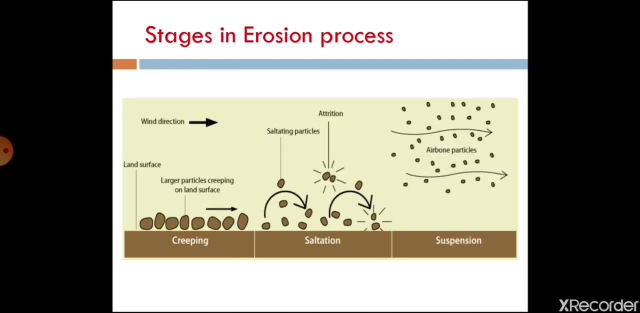 reduce and automatically the soil particle will drop down from the flowing wind and it will deposit somewhere. now if we want just clarify all those think particle, there are few kind of particles which are moving along with the air or wind. so if we'll see which kind of particle, so obviously. 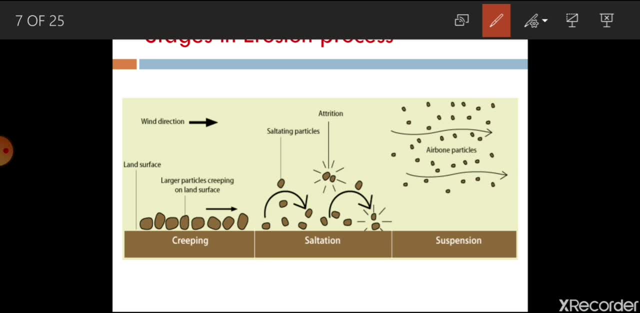 there may be a few particle which are, which may be in larger in size. few particles may be in in lesser size or few particle. you very fine or very fine particle or you can say very minute particles are there into the wind. so this slide categorize the all the particles in three category, that is, creep, saltation and 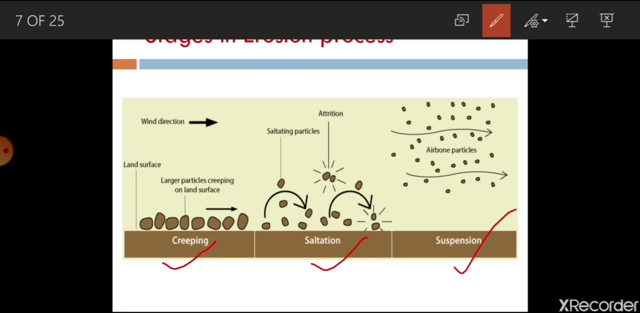 suspension. so creep is that particle or creep. creep is considering those particle which are moved over the surface onto, which are moved moving on the surface due to action of wind. say, this big particle are detached by the force of wind. now, due to force of wind, this particle will roll down here here and here here, like that. similarly, 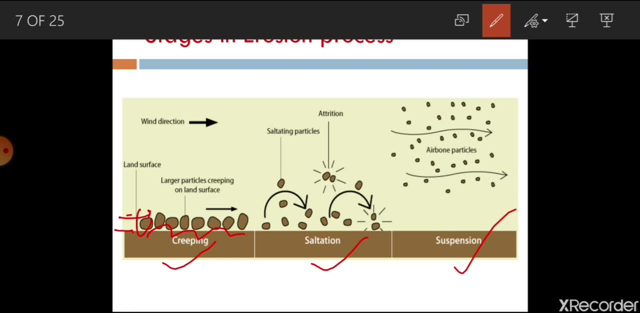 similarly, different particles are also detached from different places of the field and it is moving like this: these are different particles, which is moving, but it is not lifting, it is just dragging onto the field, so it's called creeping. now, when such particles, there is a possibility that not. 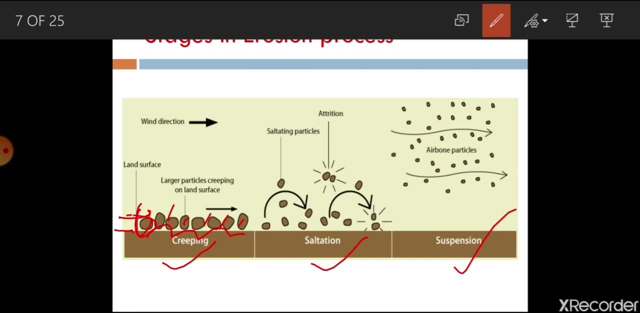 necessary that every time large particle will detach, there is a possibility few particle lesser in size will detach. so they will move. but due to effect of wind, due to velocity of wind, there is a chance that these particles may jump and then jump and then drop, and then again force of wind will come and then again jump and drop. so 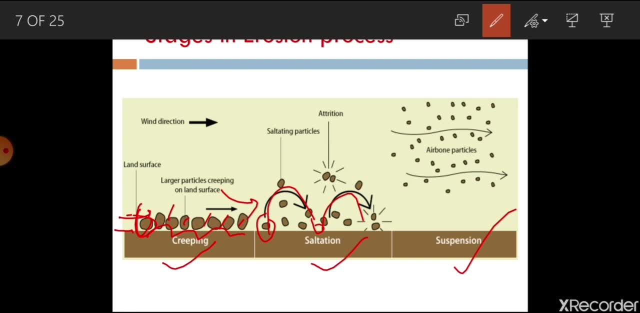 this moment is involving jumping a few minutes. sometimes it may lift. it will go at certain distance, then, due to uh velocity potential, it will drop and then again it will lift and don't go ahead. okay, so such kind of uh phenomena comes under salting. there is also a chance of movement of particle by striking, say. if such particles are moving and 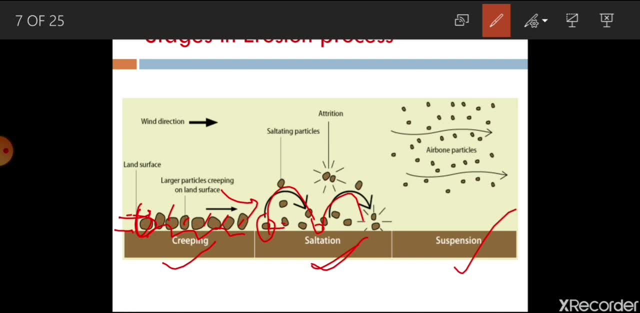 this particle is striking to this and it is going ahead, so this is also comes under saltation. now there is a possibility. another possibility is there. these particles may hit each other and become two parts. so this is also a possibility, that such particles may hit each other and become two parts. 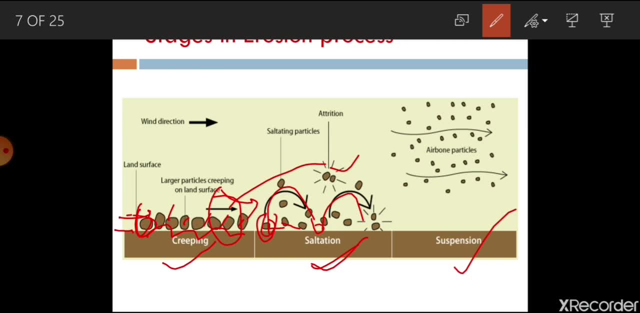 like this, or when such particles are jumped after striking onto the ground. there is a possibility it may. it may become two part or two particles. so due to this fraction, a fine particle is removed, a fine soil particle is removed, so that fine particle is not sufficient or not heavier enough to 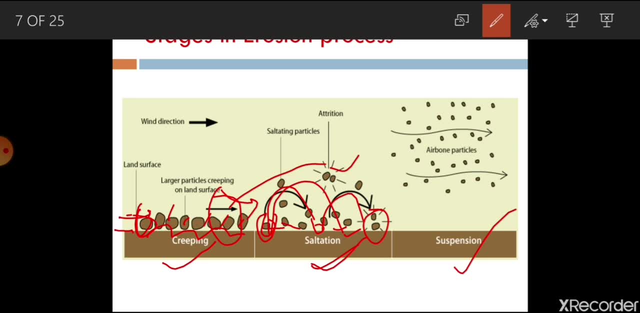 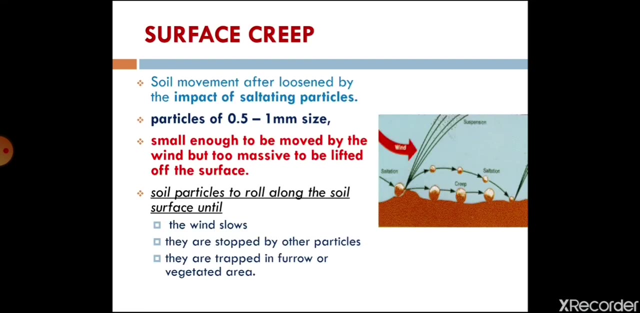 be on the ground surface. okay, so what will happen? this lighter particle will move into, will flow with the air or wind and it will be in suspension mode. so that called in suspension. so if you'll see individually surface creep, consider the soil particle of size 0.5 to 1 mm- little bit higher size. 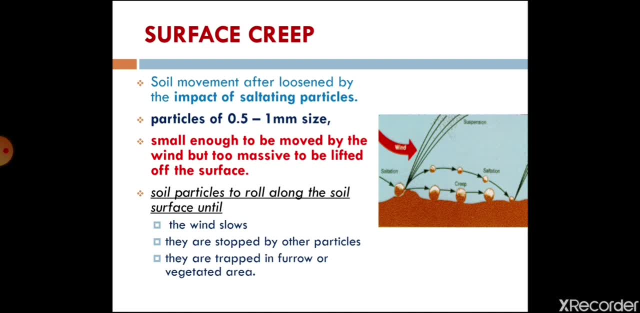 okay. and the soil particle to roll along the soil surface until the wind slow they stopped by other particles or you can say like a physical barrier or trapped in furrow or vegetative area. so these particles are enough, small enough to be moved by the wind, but too, you can say, heavier enough to lift by the air. that is surface. 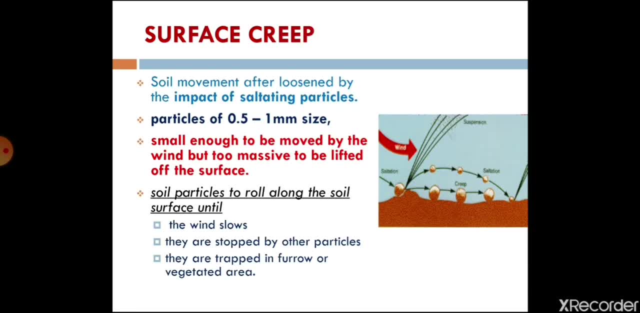 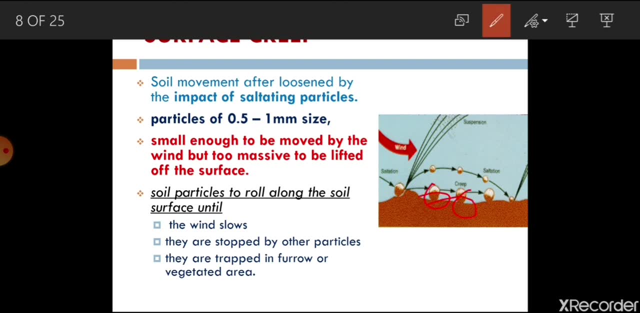 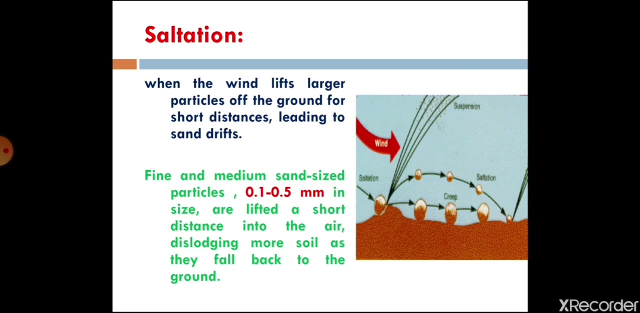 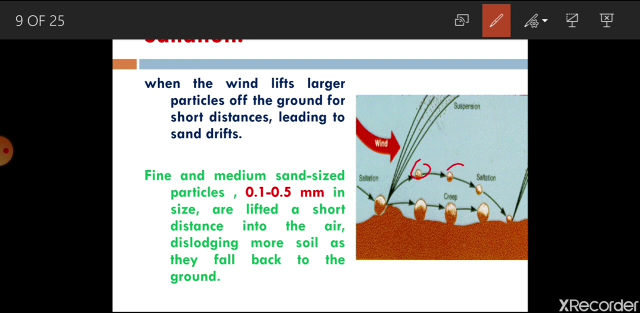 creep. so here you can see this big size. the bigger one is under surface creep or creeping. now, saltation, when the wind lift larger particle of the ground from the short distance, means these are the smaller particles, these it is jumping from under the surface and some smaller and longer particles are attached into the surface. 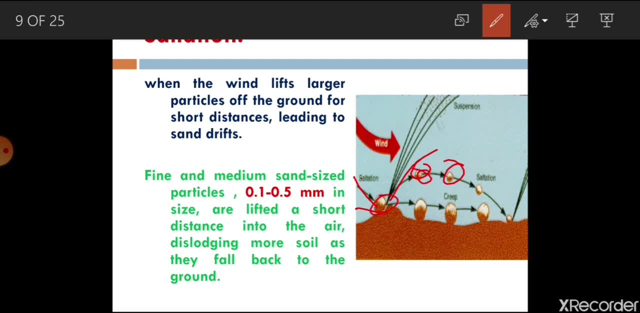 through the surface it will come under fold. or exemple, the wind. there is a wind striking for theữa, the wind striking here, and due to this strike some larger particles, some medium particle or some here minute particle will detach, so and few particles will be in suspension mode, so that will be in suspension. so in case of 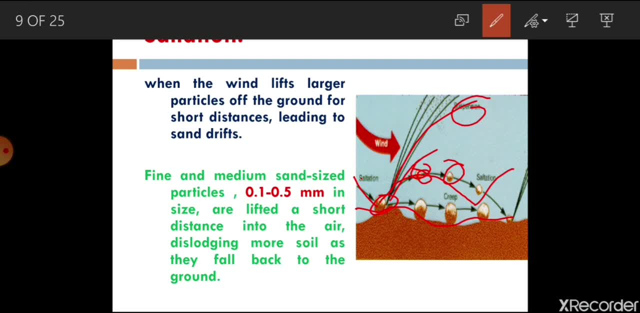 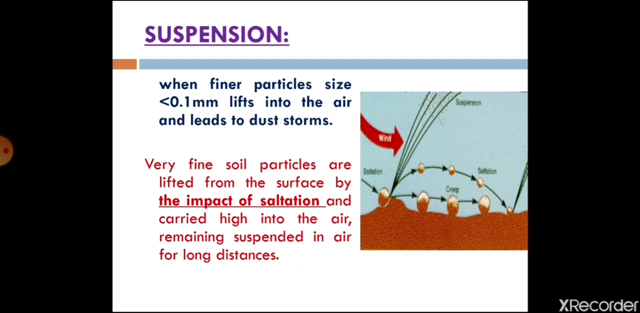 suspension. the particle size are ranging from 0.1 to 0.5 mm. okay, and comparatively it will cover the more distance than the creep surface creep, whereas it will be, it is covering distance very lesser than the suspended particle. now, suspension: very fine particle which is having 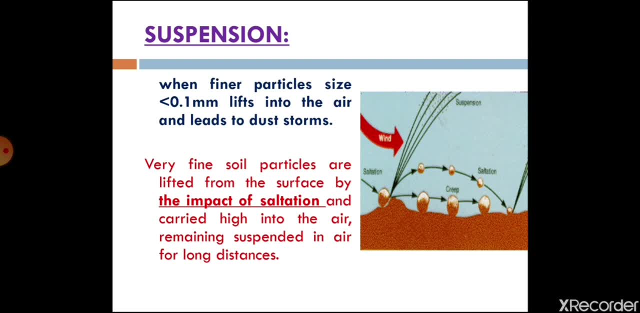 the particle size less than 0.1 mm and due to wind velocity or due to force of the particle size, it will cover more distance than the suspended particle of air. it will be in suspension mode okay and that suspension- a particle which is suspension may create due to impact of saltation or wind, may erode the fine particle. 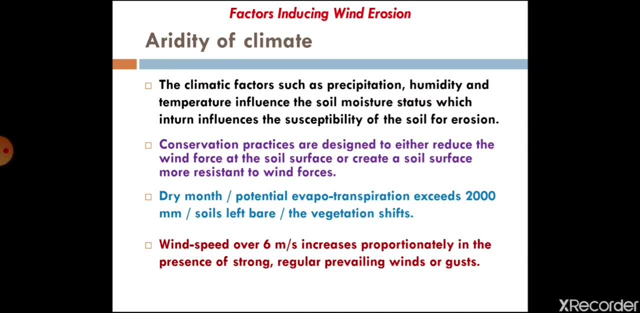 now. now there are few factors which is affecting the wind erosion, so the major factor are climate. climate includes the humidity, temperature, rainfall and other soil parameters or other climatic parameter which is affecting the soil parameter, like moisture contained, crop, residue, stubbles available onto the ground. so these are such factor, the presence of these factors. 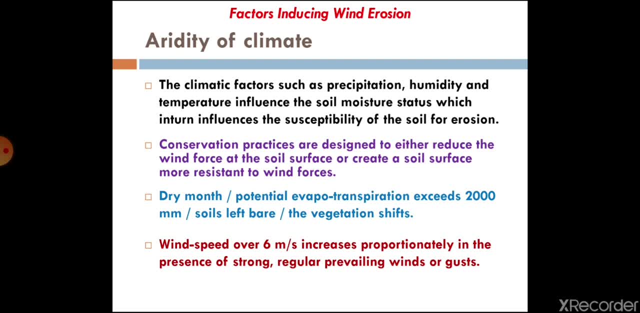 affecting the amount of wind erosion. so, for example, if you have a wind erosion, so usually, lets say, if rainfall is continuous, and in high rainfall area, soil moisture tends to be higher, so there is, in such cases, very less amount of wind erosion takes place, or there is less chance of wind erosion. similarly, in low rainfall area or area where precipitation 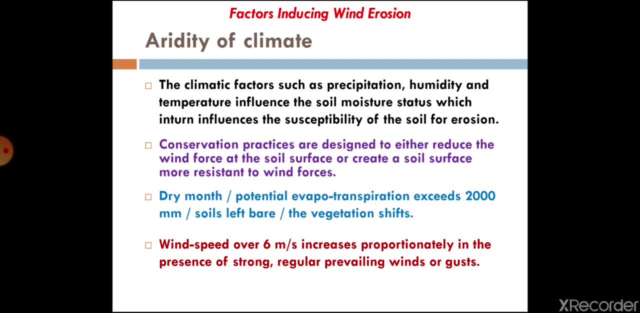 is low, rainfall is low. so at the time of rainfall or few months after rainfall, when moisture contained of the soil within the limit when wind erosion, wind erosion will be limited. but in case of dry month, when rainfall over rainfall season is gone and then high temperature creates the 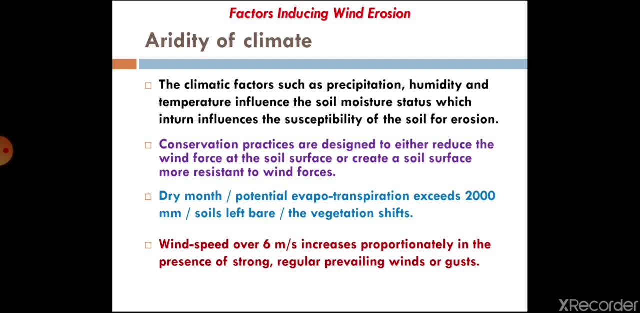 high temperature removes the moisture contained of the soil and that particular type. at that particular time the soil moisture will be less and if soil moisture is less that means binding property of soil will be less or will be weaker and that moment when wind flow it has more. 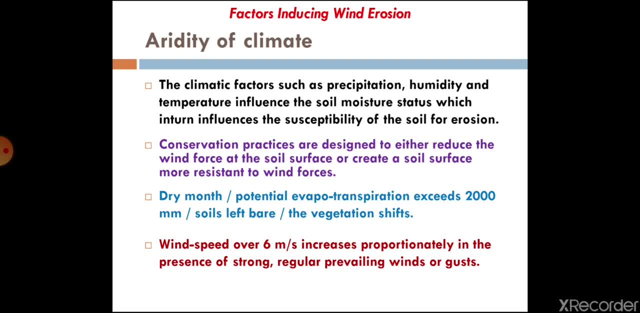 susceptibility or propensity to detach soil particle and it become. it turns into wind erosion. further, if you see, evapotranspiration rate exceeds more than 2,000 mm in dry area. in dry area or you can say in dry month. similarly, conservation practices: if conservation practices are adopted into particular field, so there will be a less chance of wind. 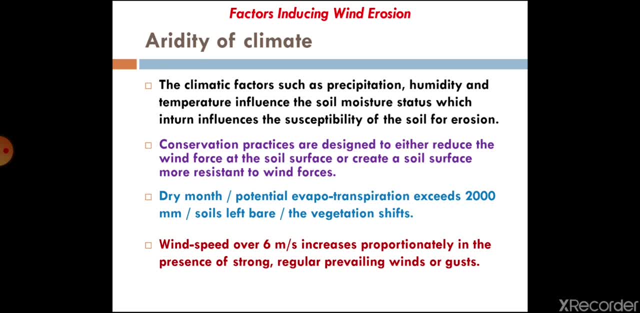 erosion, because conservational practices are acting as a physical barrier against the wind erosion. so as well as if we will talk about the wind speed, so beyond these 6 meter per second, there is a very high chances of erosion due to wind. such kind of wind speed may create swirling. 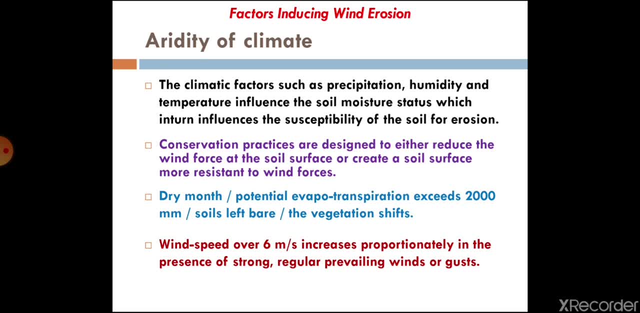 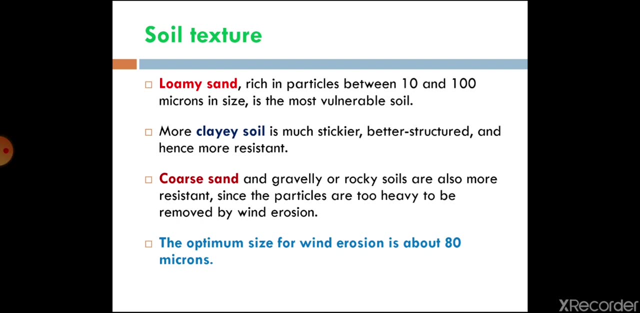 movement gurds, and you can say eddy, so that the lifting of soil particle is become easy. so now the another important. I talked about the soil parameter. so if we will see the type of structure, sorry, if we will see the type of structure of the soil, so in case of loamy, 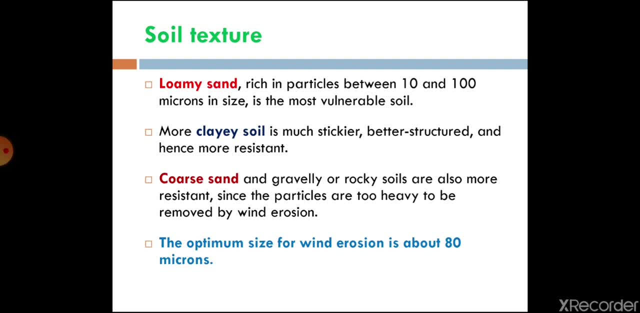 sand where loamy sand soils are available, into the field. so you know, the loamy sand are available, the particle size available in 10 to 100 microns, and very fine. these are the very fine particles and such fine particles are easily, could be easily eroded by the. 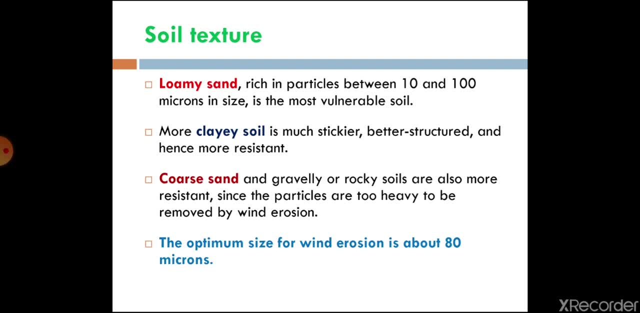 wind. similarly, if we talk about the clay soil, clay soil has one good property against for the wind: erosion, that is, stickiness at at some moisture content, or it is bad, best, or you can say better structured clay soil is better structure. so due to moisture or due to water present into the clay soil, it is showing more. 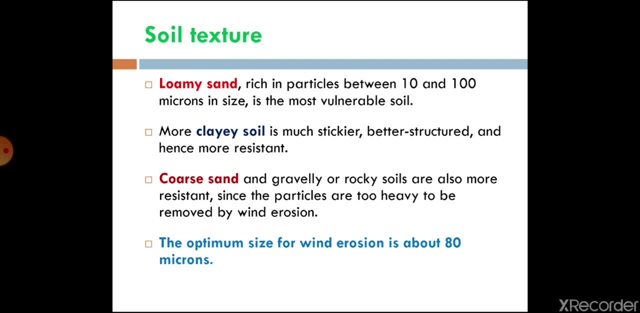 resistance against the wind erosion. so it is better for the field where clay soil is available now coming to the chorus end, and gravel sand or gravel soil. so in chorus sand or gravel soil there is a one point that this particular soil may be available with larger particle size. so when particle size is heavier, 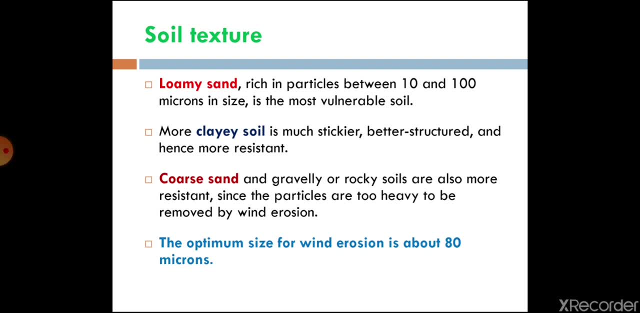 so there will would be a less effect of wind erosion because particles are not able to lift by the wind forces at very high extreme cases, when wind is flowing at very high speed, then only such particles will move or will under creep or particle suspension saltation, you can say. now it has been found that the most susceptible 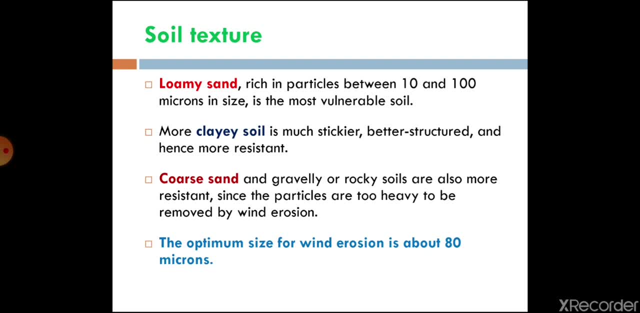 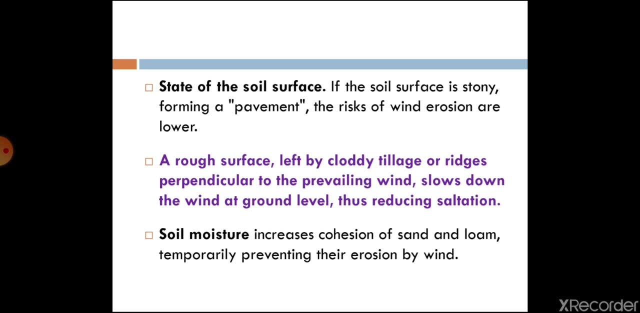 soil particle size is about 18 micron, which is much more set up susceptible for the wind erosion. now, if soil condition are rough, tillage practices are there onto the field. so tillage practices loses the soil due to wind, due to velocity of wind, the fine particles 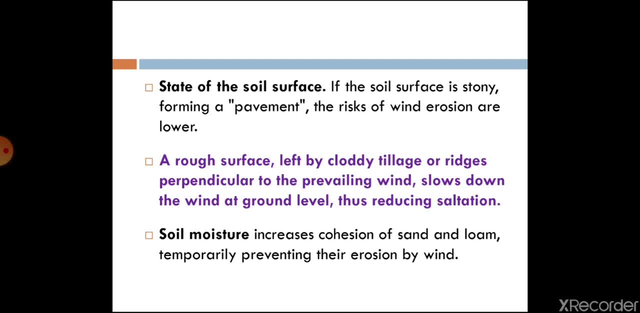 or pulverized particle. pulverized soil may have chance to lift and it will go along with the wind. so in case of field where tillage operation has already been done so that particular village, that particular field would be more susceptible for the wind erosion. and then moisture content we have already discussed: if we increase soil moisture, it 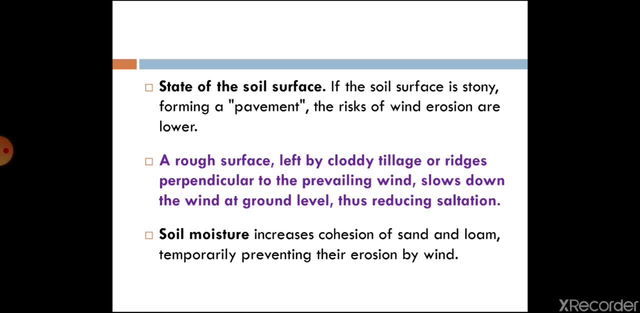 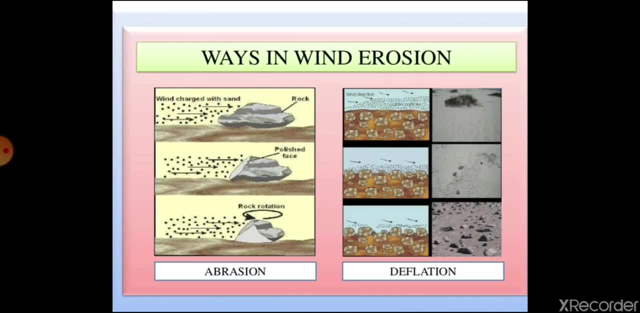 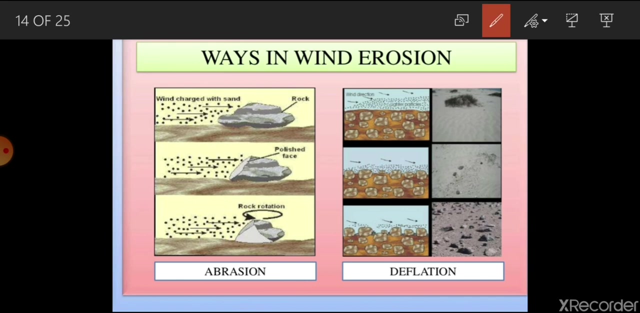 increase the cohesive and adhesive property of soil with and stubbles, so there is a less chance of erosion. now erosion could be of two types. basically, one is abrasion, another one is deflation. abrasion includes the airborne particle. if you will see, these are the wind flowing, and this particular wind is not only the air alone. it has some 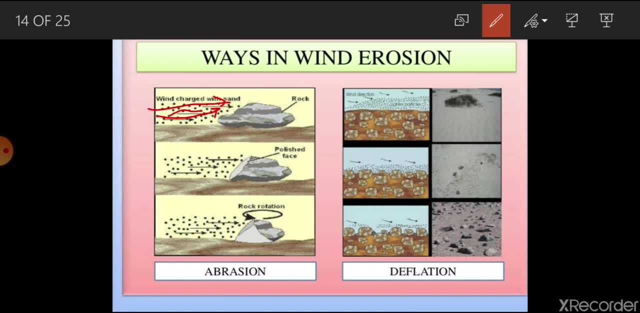 airborne particle, suspended particle, when such a suspended particle striking to some physical barrier- or you can just consider this is a rock, and when such airborne particle is striking onto the surface of rock gradually, after some time, after some year, there is a chance that such rock may get eroded like this. you can observe the face. 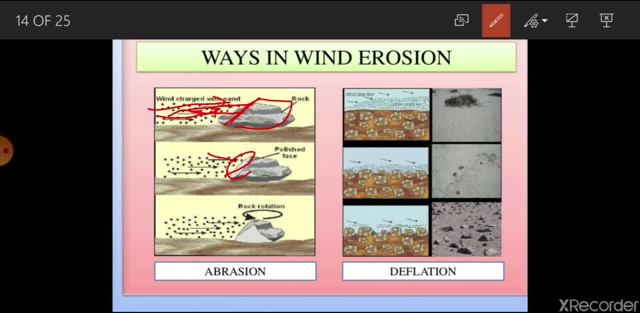 of rock and as time passes, this particular area would be, would be eroded. so abrasion includes the kind of erosion which is done by the airborne particle, whereas deflation in includes the moment of fine particle, say, for example, for instance, the moment of fine particle. say, for example, for instance: 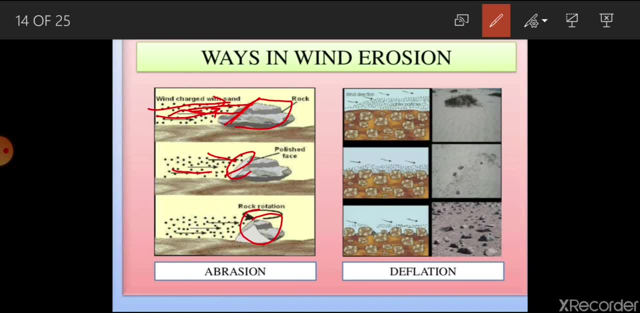 say, for example: for instance, you can see your field is covered by the fine soil over the top and then under beneath of this, some larger particle are there. so when wind flow from direction, what it will do? it will erode the top soil. first it will move the fine particle from, first from the top and then when 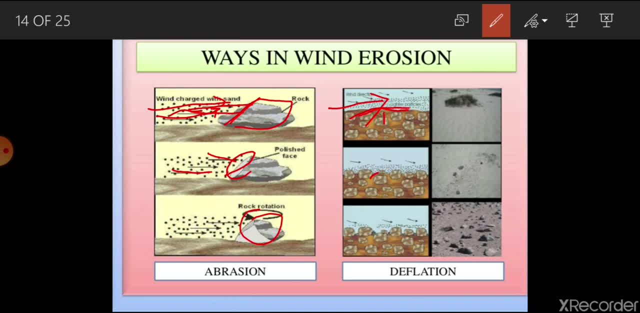 top layer is moved, then few particles in between the these larger particles are kept. so then continuous wind movement will displace such kind of fine particle too. okay, now field is available with only larger particle, and this wind is not able to move such kind of heavier particle. so 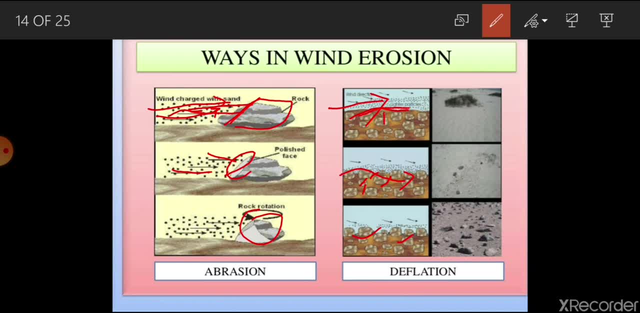 this is the deflation deflation. deflation, where wind velocity moves the soil particle and soil vertical and the affected area will be like this, whereas abrasion includes the erosion by the moment of airborne particle and area will get eroded. so these are the basic, the two difference in, two difference in. 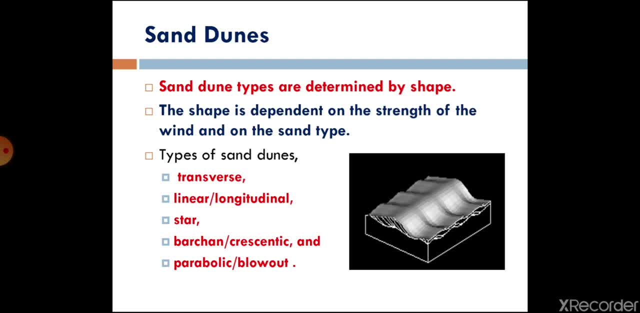 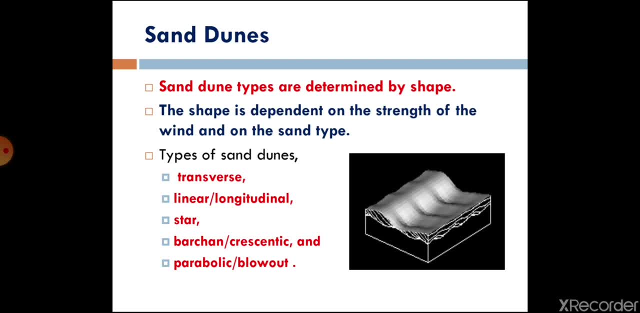 area. so it is creating some kind of structures called dunes. so dunes are large mass of wind blown sand. it is the most common in desert area, particularly in Sahara and Registan, particularly in Rajasthan, India. okay, so these are the biggest structures which is created by the wind. so if directly, if we'll look. 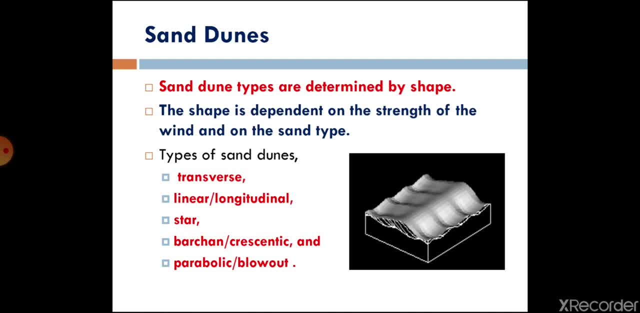 into the sand dune. so sand dune is a mount or hill or ridge of sand formed by wind, usually along the beach or in desert area. dunes form when blow sand into sheltered area behind the obstacle, and it particularly grow gradually as grains of sand. 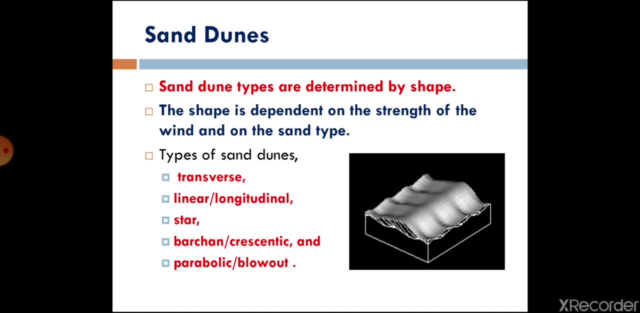 accumulate at particular area or at particular place and if you'll see the Dan dunes, every dune has windward side and slip face. so, for example, and particularly most of the sand dunes are recognized by the its shape and different kind of shapes of sand dunes form. 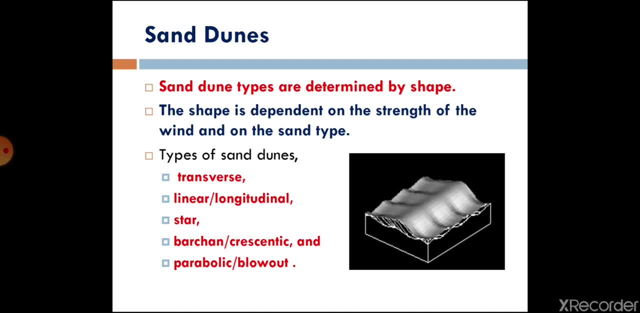 are formed based on the strength of wind, velocity, okay, and different kind of shape. I will come into them. I will show into the next slide. so what are different kinds of sand dunes? they are. they could be transverse, longitudinal, star-shaped, bark and shaped or parabolic shaped. so these are the few types of 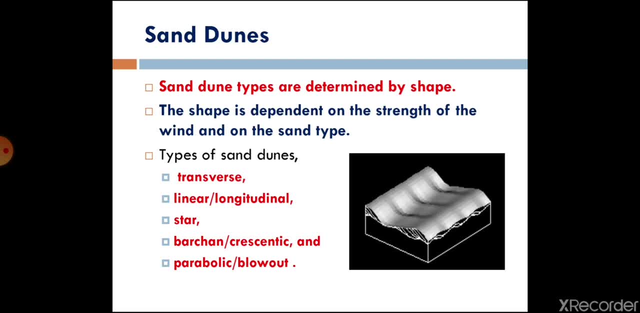 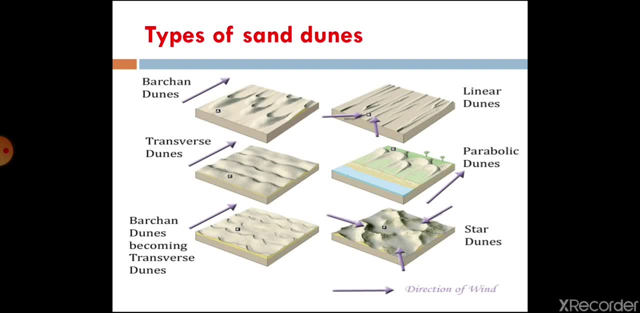 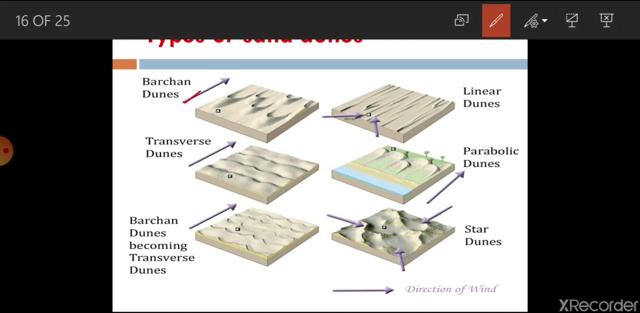 structure or types of dunes, which you can see in this slide. okay, now see, all kind of dunes are differing in their shape. so if we'll see the first one- bark and dunes- here you can see the wind direction. wait, this is the wind direction. this is the wind direction. so now, when wind is blowing, 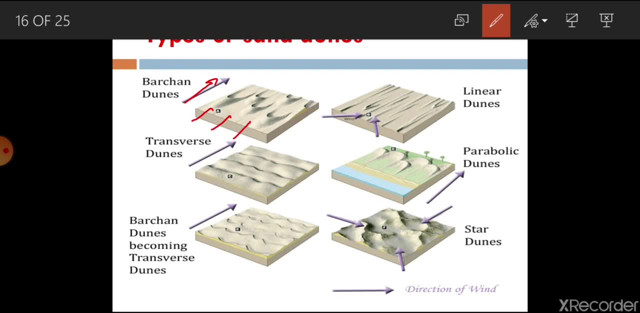 okay, from a area of desert, it is creating such kind of a structure, this where one part is convex and another one either. another part is concave, so convex side is a side along with the wind and convex- sorry, concave, concave side is up in the 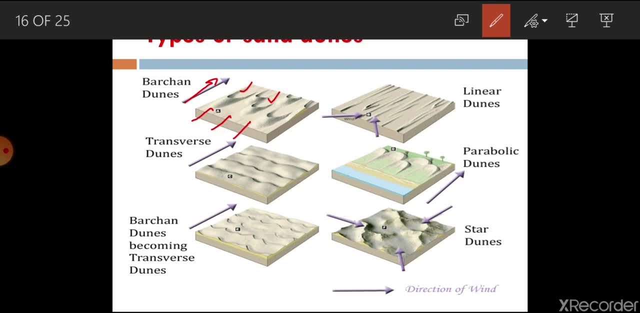 direction of opposite of wind blow. so basically, when such kind of Prophet has opened, Freelander follows and it is entste damage in the direction of your left hand, for the very left hand are given theточka Hi. i know i have explained that in the previous slide. 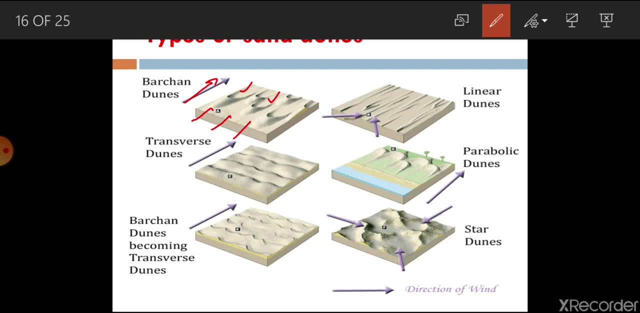 but when you move to corner on to this side, it goes left. when you push here it goes right, and so on and so on. and initially because people has picked up, and so in the connection line we have theune shape, we have kinetic shape. this shape now is separated from the Coin. are 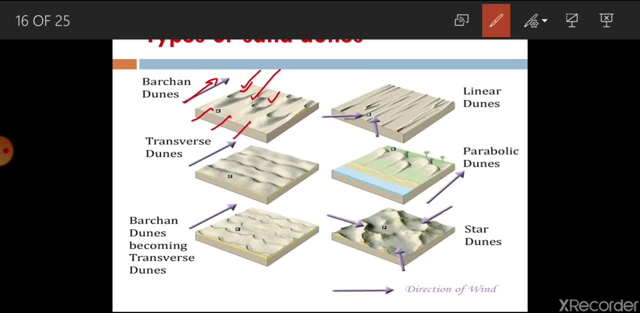 two directional wind, or you can understood: one wind is coming from this side, one going so, and they both mix and go in straight. so due to such, some linear dunes are being created. similarly, when wind velocity or a strength of wind is in in variable condition, so the sand initially. 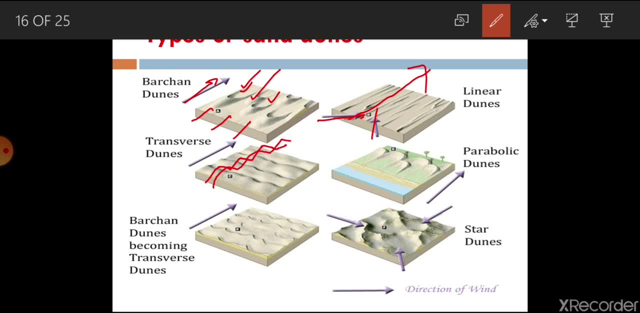 form, such kind of transverse shape, or you can say it's a across the direction of wind. it is forming across the direction of wind, whereas parabolic shape, particular parabolic dunes, are specific to the wind, so it is in variable condition. so it is in variable condition. 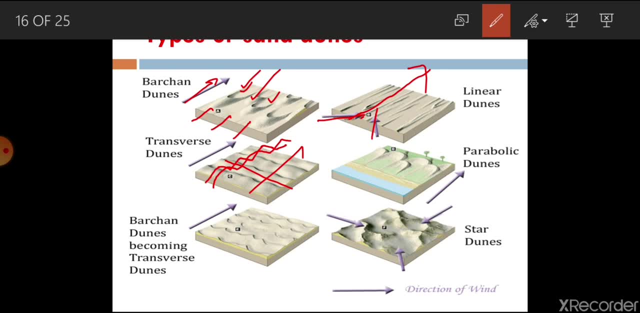 specifically in coastal area, where tides or you can say high wind, high wind flow is coming from this direction, from sea direction, and it is creating such kind of structure. this particular parabolic structures and parabolic dunes and bark and dunes are similar in shape or looks like similar, but basic difference in that the bark and dune has 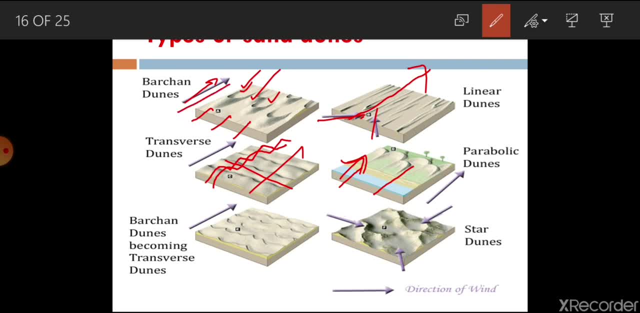 convex shape along the along the direction, whereas here it is in opposite direction. see, so these are the basic difference in the bark and parabolic. otherwise they looks like same, only the direction is the difference. and now a star dunes. star dunes are formed due to multi-directional wind. 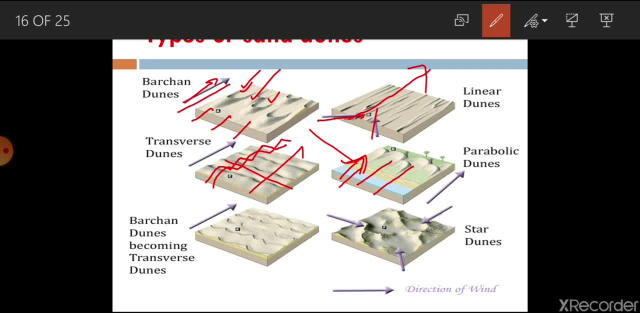 and due to this number of when, winds are coming from different direction, so sand are being removed from the bottom and all these things are, or you can say the center is becoming high and other slip phases are becoming down or concave side, so that time of the such kind of structure known. 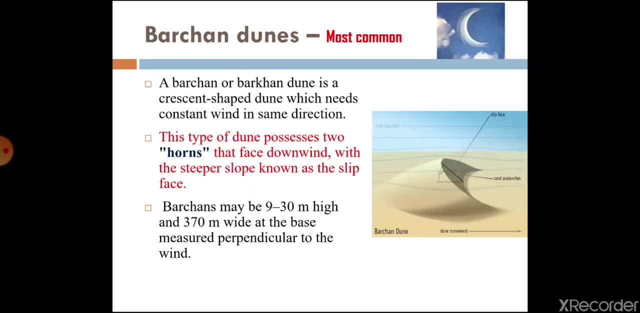 as star dunes. so, individually, I will see. what is this bark and dune? yes, it's just like a half moon shape and you can. I already informed you that any kind of dune have two specific parameter or specific shape, that is, windward side and slip phase. so you can see, this is the slip phase. 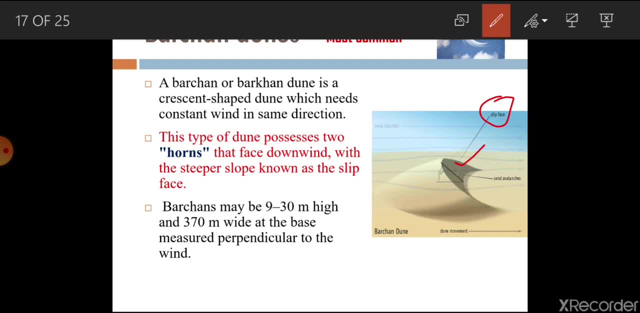 this is a place of bark and dune and this particular angle is generally varying 30 to 34 degree. this one, sorry, yeah, this one you can see here. okay, this is slip shape, this is concave side, this is convex side and wind is flowing from this direction and these two, this is this length is becoming long. 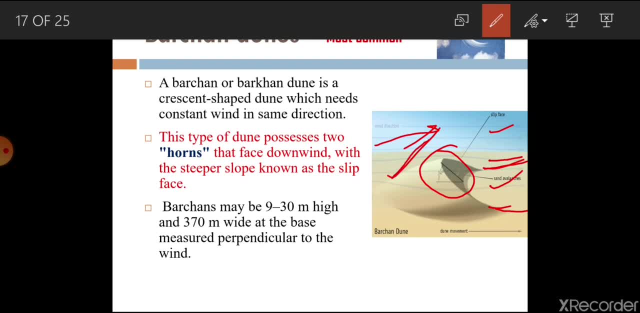 longer, and when wind is coming like this, it is going here. so these two are calling called as a horn. okay, now the physical structure, or you can say the specification of bark and dune are generally 9 to 30 meter height, the, and it may have width of nearly 350 to 400 or. 구독 muita peế możemyете. 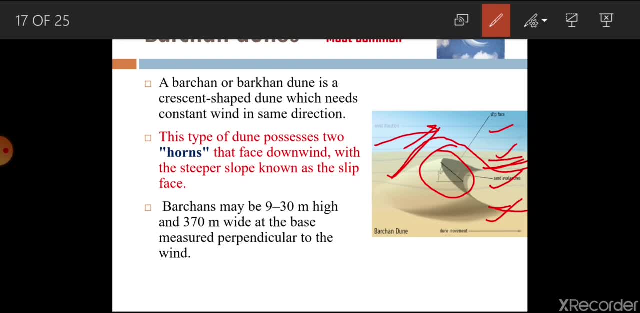 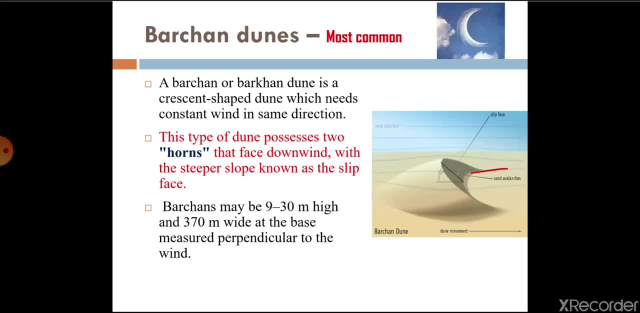 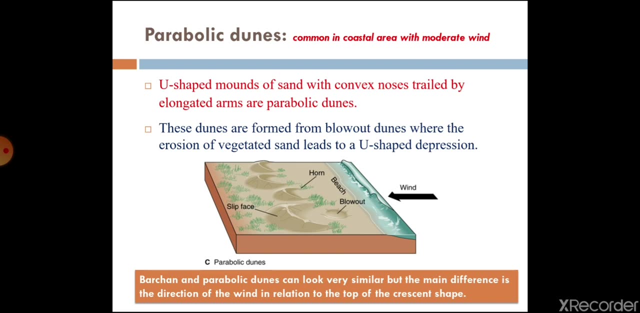 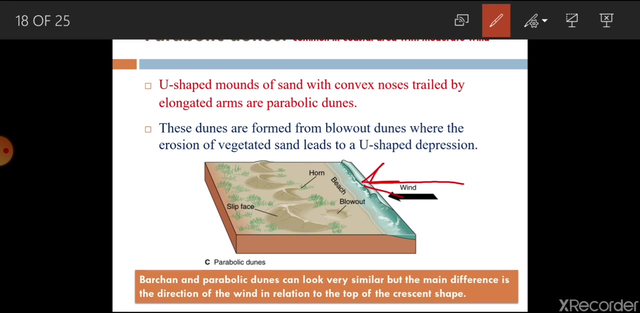 dekorasiye to 370 meter wide, Now parabolic, similar to Barken, but direction of wind is from this side, from particularly. it is formed particularly in coastal area and when wind is striking to the sand or to the field of surface of the coastal area it creates such kind of shape and in this 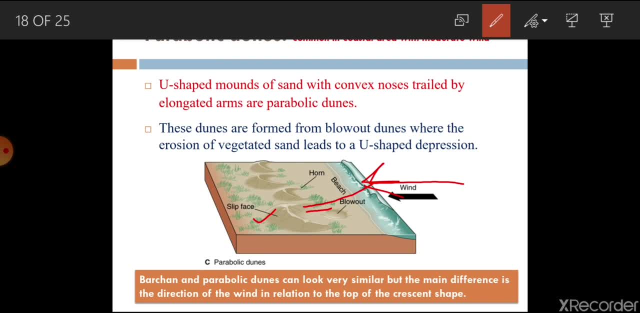 particular, this convex side is slip and this one is windward side from here. So these dunes are formed from blowout dunes Where Erosion of vegetative land leads to U-shape depression. and yes, here it is written. the Barken and parabolic dunes look similar, but the main difference in the direction of wind. 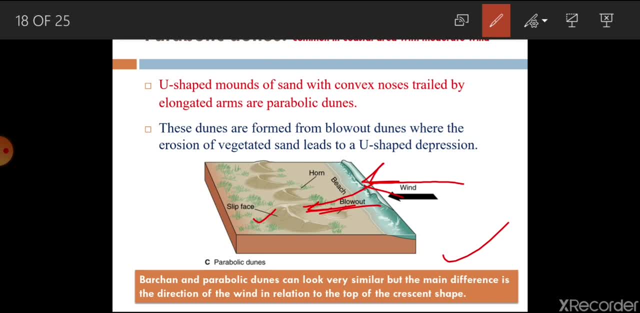 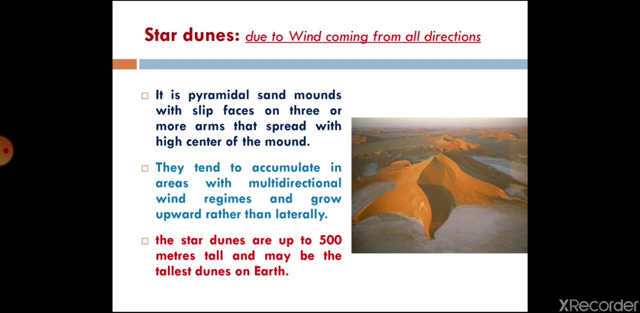 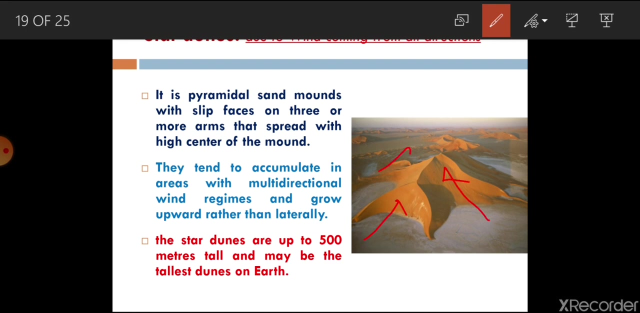 in relation to the top of the crescent shape. Now Stardune. Stardune is due to multi-directional wind, So just see. Okay, Just a minute. Yes See, One wind is from this direction. another one is this: 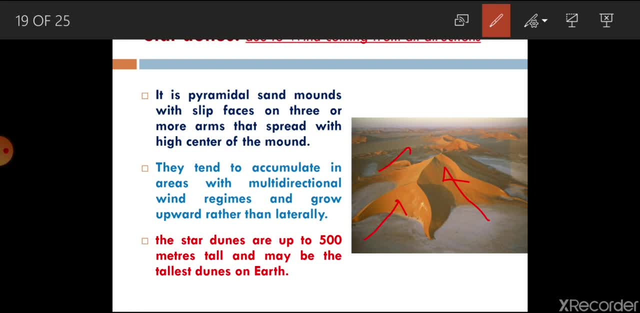 So it's a kind of pyramidal shand mount with number of slip faces. They tends to accumulate in area where multi-directional winds resumes and slowly, slowly, its center is becoming high, Reaching at height, And this particular center from the bottom may go up to 400 to 500 meters. 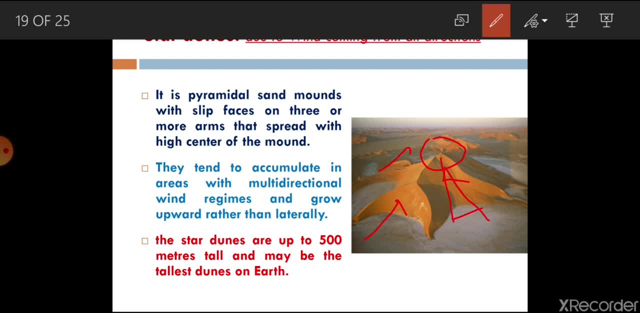 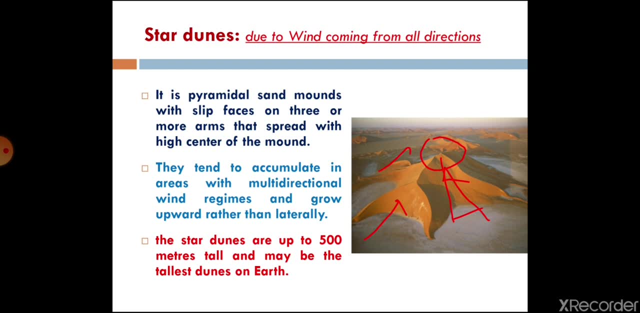 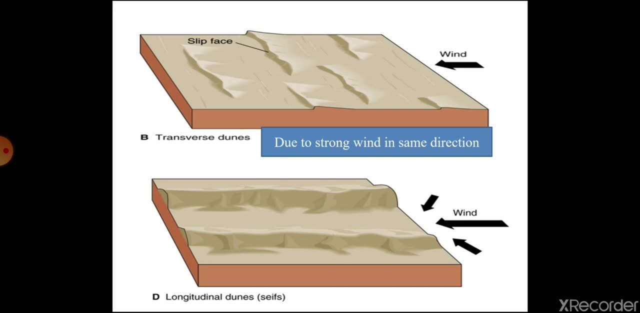 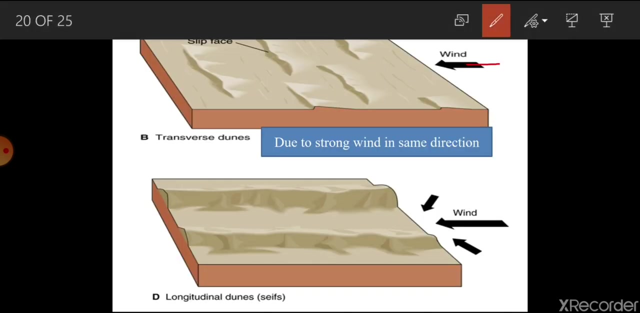 Okay, So this is the multi- sorry, it's a Stardune created by the multi-directional wind. Now, similarly, you can see transverse dune. Okay, Due to strong wind in- sorry, in linear direction. This, so this at such particular point. if wind become weaker, so sand deposit will take. 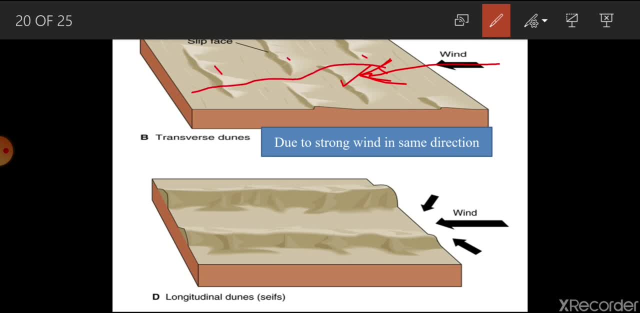 place and then further. so this is how slowly sand dunes is created here, Now longitudinal along the wind. So you can see that this is not only wind but partially similar winds of lesser intensity than the main wind, For example, if this center one is the wind velocity of higher magnitude and it's joining. 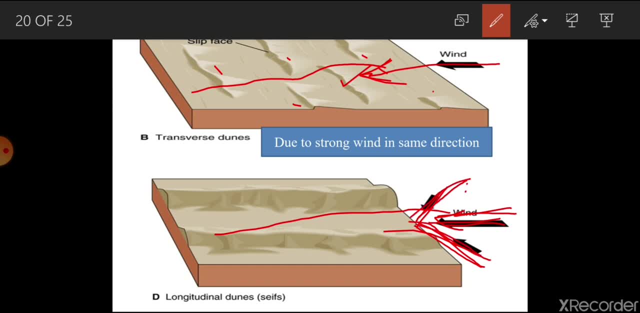 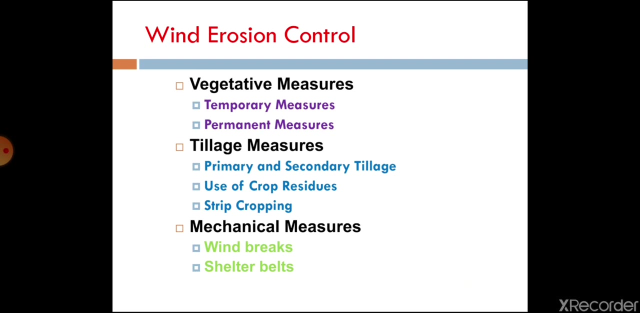 the it is two other winds are joining at this particular place and then it is moving. So what happened? Due to this longitudinal, Due to this, longitudinal dunes are created So to minimize such kind of effect or to minimize the wind erosion. there are three major three. 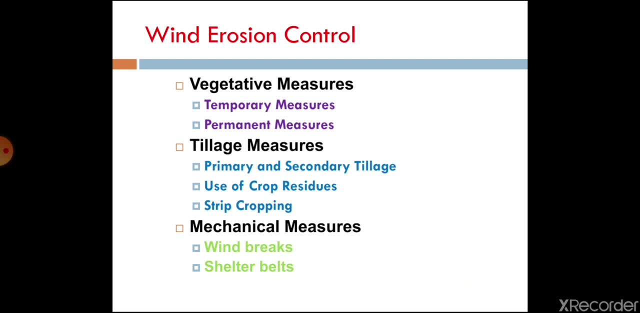 measures to control the wind erosion. So they are the three measures. One is vegetative measures, tillage measures and mechanical measures, Where vegetative measures, Vegetative measures, could be categorized in two way: temporary and permanent. Similarly, in tillage, primaries and secondary tillage, operation or crop residue could be. 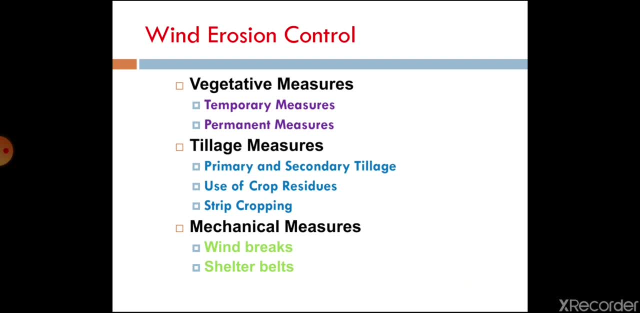 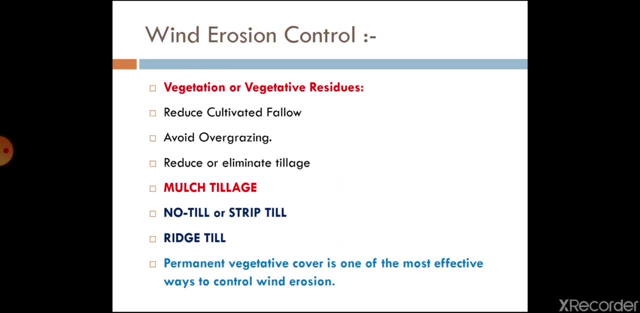 and shelter belts Now similarly, under those conditions only. I'm briefing In very brief. I'm just explaining you In vegetative measures. you can grow vegetation. you can have a field crop on the land surface. don't do tillage operation, avoid over grazing. 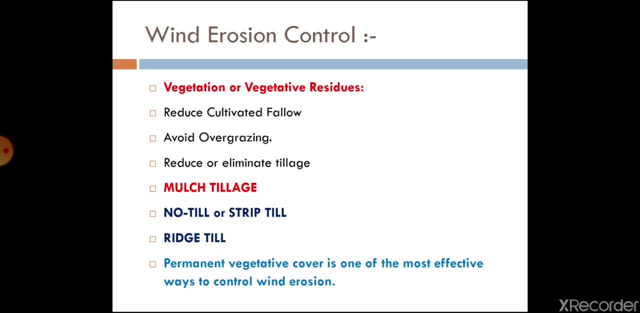 of the animal, so that soil may not be available in lozenge form and that particular time your wind velocity or wind erosion may be reduced. similarly, some other kind of method like ridge tillage or strip tillage could be utilized where strip of land could be cultivated and rest. 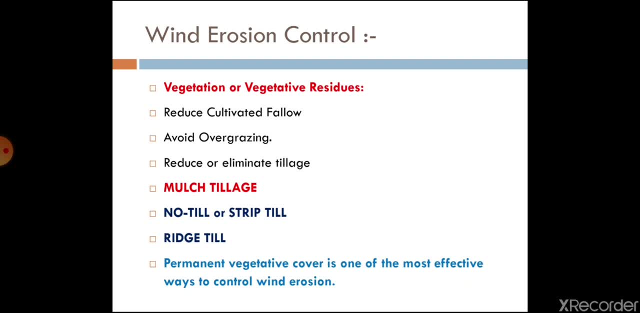 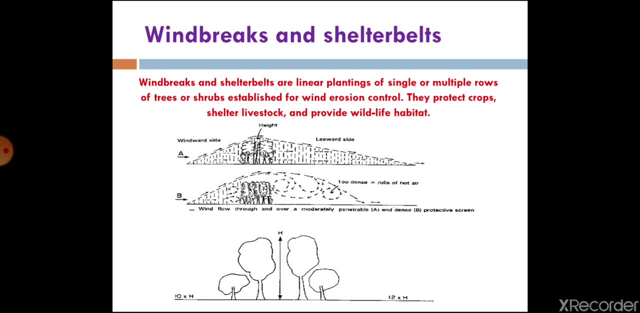 of the field left undisturbed. so this is the few methods where you can apply your situation and you can do the practices. you can reduce the wind erosion. now, another method are wind breaks and shelter bed. yes, i am starting another, you slide, just wait. so wind break and shelter beds are the linear planting of single or multiple rows. 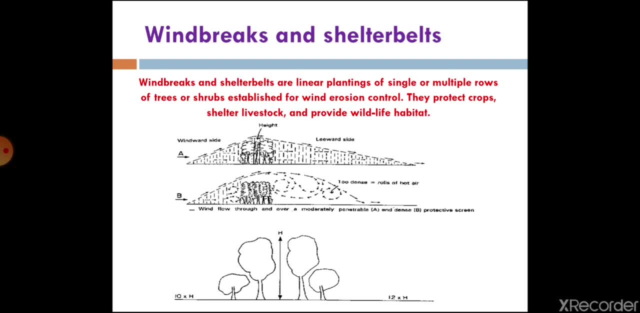 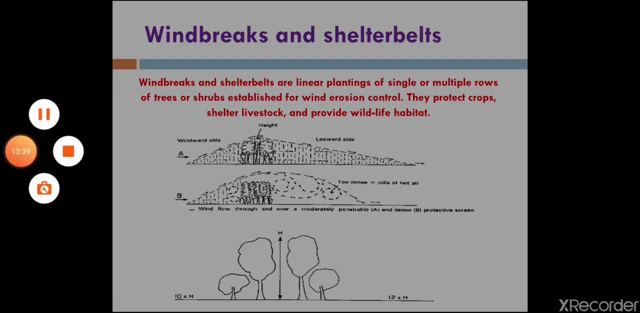 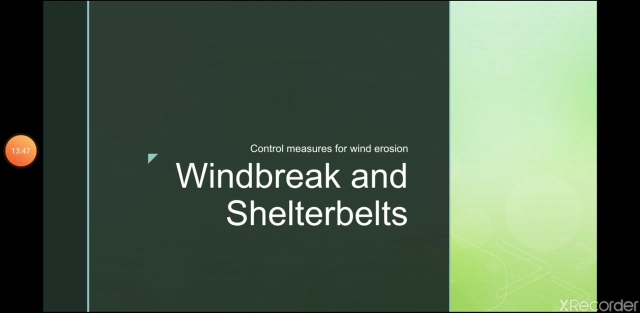 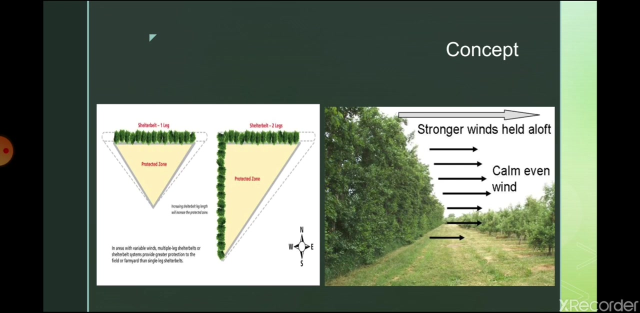 of trees or shrubs established for wind erosion control. they protect crop, shelter livestock and provide wildlife habitat. so what is this actually? i have another slide, i am just explaining you wait. so for controlling and reducing the impact of wind erosion, shelter beds are effective ways. so here you can see: shelter bed is a line of tree or shrubs planted to protect area specifically. 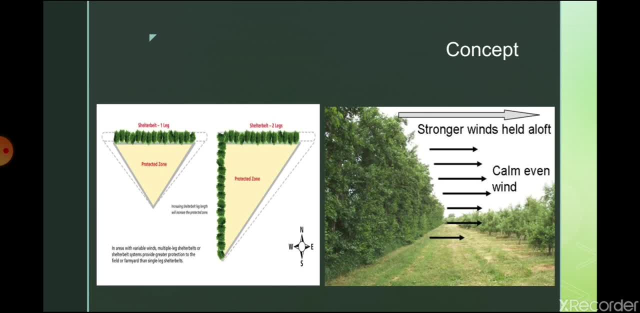 a field, field which is available with crop. okay, so in this particular diagram, you can observe that this is theном one. strachem is available from the west side. this is the number one, or one plus one or two different direction. 추석, when winds are coming from this direction, high wind, this direction you. 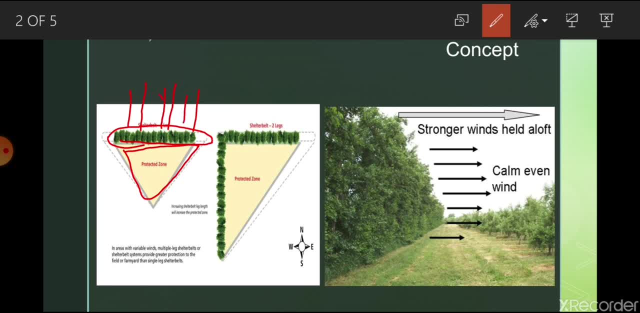 can see wind direction: high wind. so that's correct kind of direction: high wind. you can go here. this is what you are talking about. low wind in picture Forecast winds coming from prophet land is coming from this direction. our highest magnitude of that wind is particularly very high. so what will happen? this particular trees will. 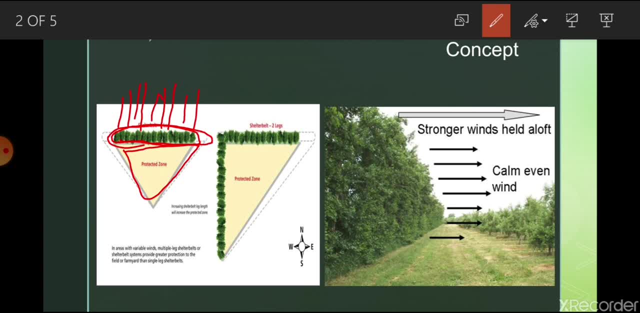 absorb the impact of, will absorb the impact of wind and it it will also reduce the wind velocity and it will allow the lesser velocity or lesser wind into the your field or cropped area, so your soil erosion will be reduced, your field crop may not be disturbed, and some other applications are similarly the. 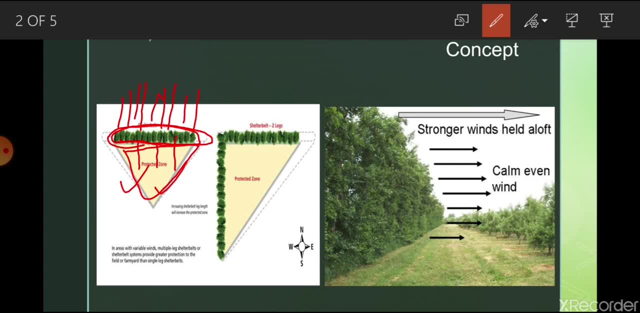 best effective way is to protect your crop or your plot, your field, from two direction. this is the best method: right angle. you have to establish, you have to establish series of plant, you have to grow a row of plants in both the direction that is, at right angle. 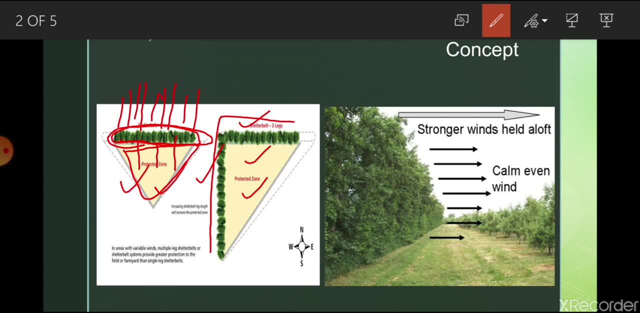 so that could save the field from wind erosion, from soil erosion, from your the disturb. it is not able to disturb your crop. so here is the practical example you can observe. see this one. this is the physical barrier, or you can say shelter bed, created by the someone. so when wind is coming, this is the 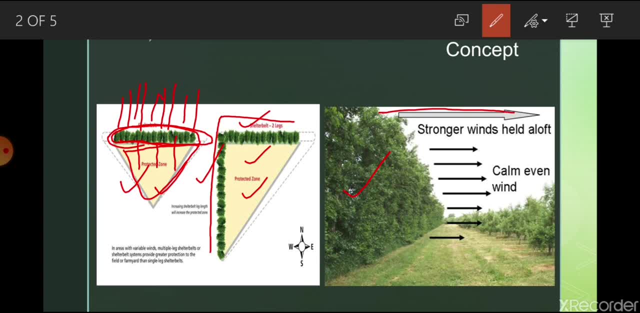 direction of wind. when wind is coming from behind of this shrubs or behind of this, you can see barrier. so it will from this, from this whole vegetation, only velocity will. sorry, wind will flow. wind will flow, but at lesser speed and that will that is not going to affect your field crop or orchard or whatever you have. so this is how the shelter 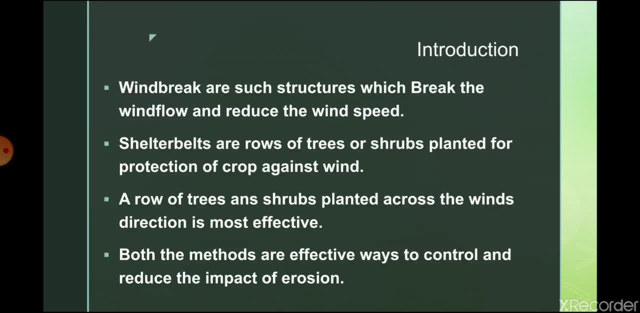 bed and wind break plays the role. so here two words are coming. one is wind break and shelter bed. so you have to understand the basic difference between two. otherwise both are similar. both are same. wind breaks are the structure which breaks the wind flow and reduce the wind. 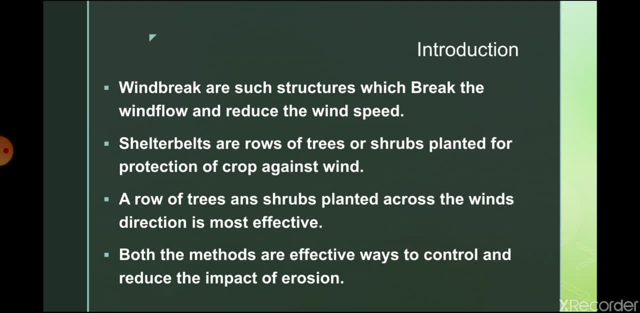 speed, while shelter, bed are the row of trees or shrubs, plants will are represented in the other ways that this pedigree is breaking the wind, so it will continue to act. the wind flow, but at lower speed. this way is the way other wind inter colors the basic process, so this is even called wind. 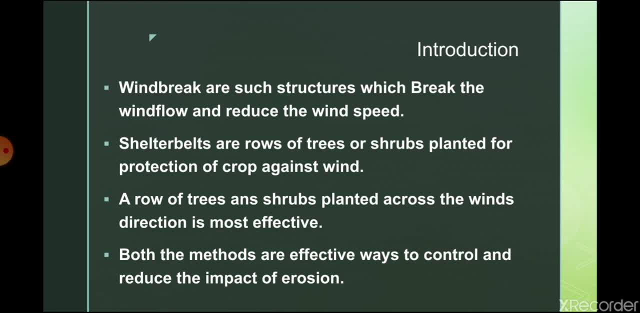 building. so, as I said, you are in flanking, but important that you are, in fact, the bigger you are in you will not get up done, but in flanking you are not going to reach the ground, the edge compared to your actual shelter bed. also, Story of Bl reactive turbojet. There are two big ways to protect legitimacy of the wind costs and solutions: body testing, partial size and, moving on to external welfare, thats what we want to change the policy of the rescue system. also, we are going to divide this into manual methods with various methods of protection. 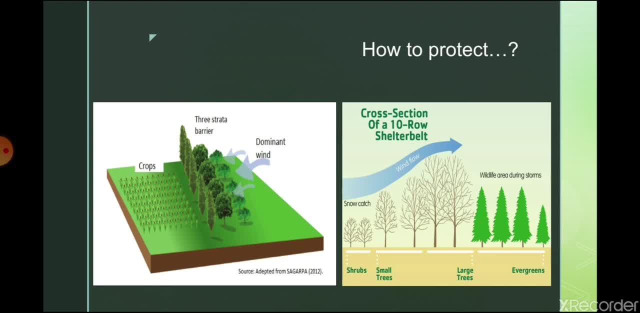 field or how to protect your surface from the wind erosion. here, see, this is your field area now. the here you can guess. let's assume this is your field area now. dominant wind is coming from this direction and this is the here is a series of, or row of, plantation, and what is the specialty? 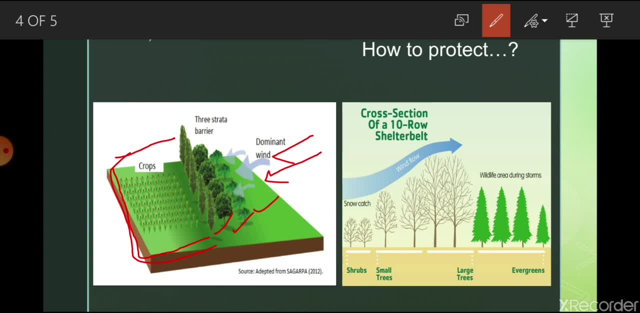 of such plantation. see minutely. observe: such kind of plants are available with shorter height compared to this. this one is little longer or bigger, and then after this is also bigger. so when wind will flow, it will pass from this, it will go up, and then go up, and when. 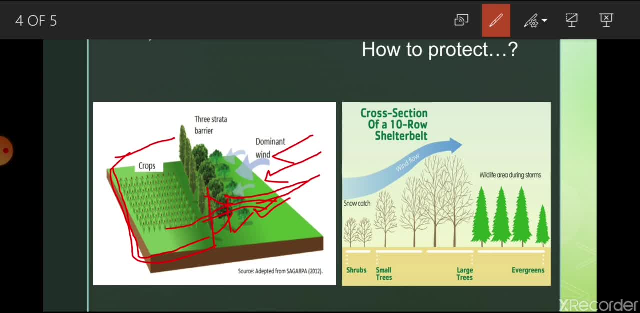 the rest. amount of wind, velocity will flow slow. amount of velocity will pass, will go through from this, but the higher amount of velocity which is coming, it will go over the field okay. so whatever wind is coming from the land, this plantation will reduce the velocity and allow the permissible rate into the your field. 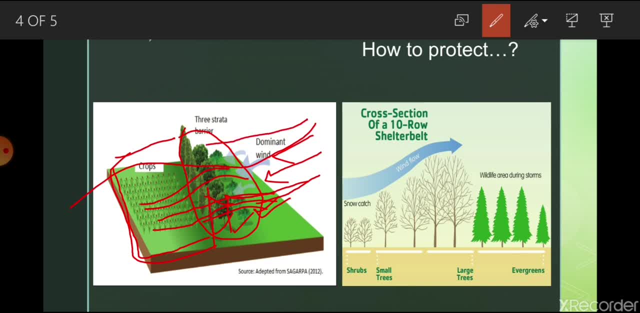 whereas wind, which is coming from over the height of this particular tree, will go straight from out from the airfield. see, this is the wind flow you can understood now: small tree, little bigger and then little, and this is your protected area. so, if wind will flow, it will go, it will cross over the field and 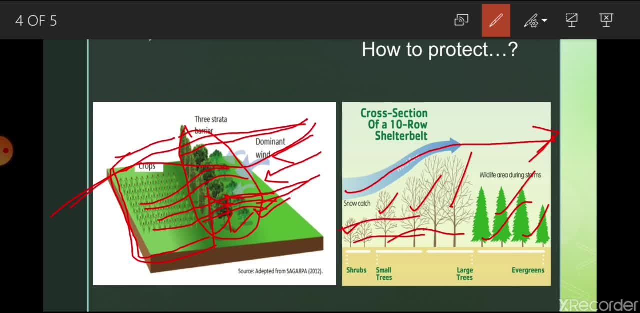 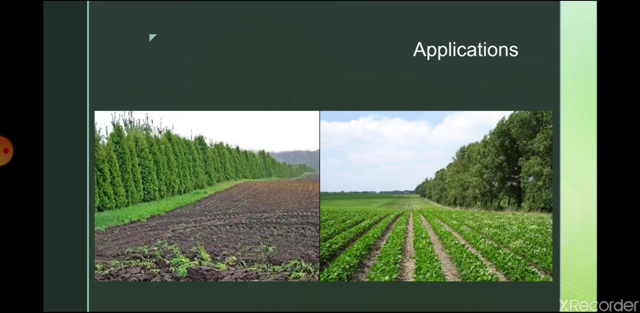 whatever weld is coming through this, it will have. it will have safer velocity. okay, so this is the you can. this is how you can establish the windbreak and shelter bed. see here shrubs, small tree, large tree, and here is your protected area. okay, so this is the windbreak and shelter.